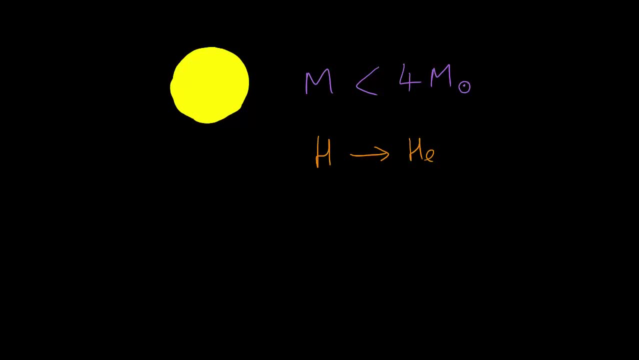 releasing energy as it does. so When the hydrogen in the core runs out, fusion will stop and there will no longer be any gas pressure available to prevent the star from collapsing. This sudden collapse will increase the core's temperature so much that helium fusion can take. 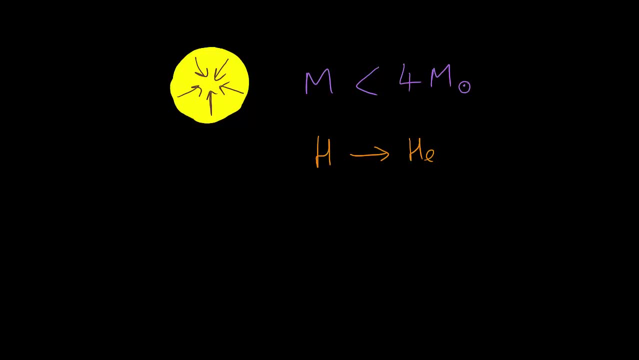 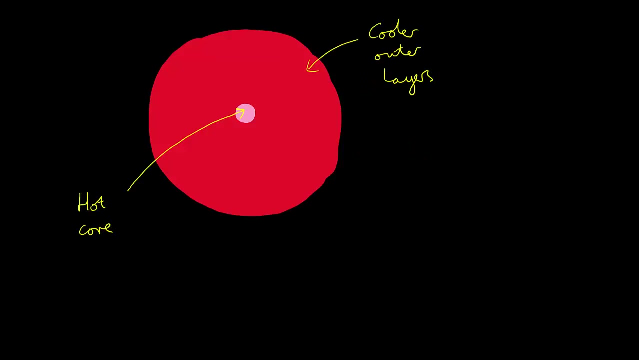 place producing heavier elements such as carbon oxygen, silicon and iron. The energy generated from this new round of nuclear fusion will cause the star to expand massively. Although it is generating more power than previously, this is spread over a much bigger area. 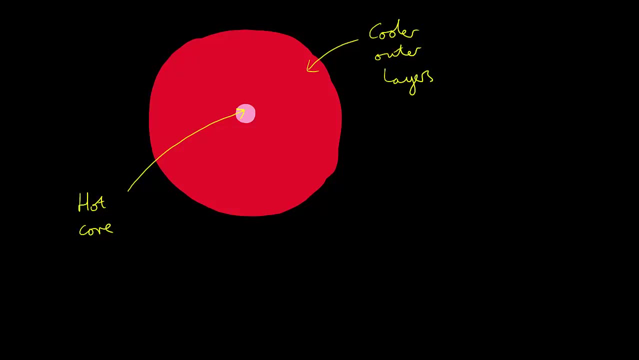 so the surface temperature is lower, producing red light. The star is now a red giant. This will happen to our sun in about 5 billion years. When it does, it will engulf Mercury and Venus and it will almost reach the surface of the earth. Whatever life forms may still be around by, that point will be finally extinguished. What happens next in the evolution of a small or medium sized star like our sun? A red giant will fuse heavier and heavier elements until it reaches iron. Iron has got one of the highest binding energies per second. The red giant will fuse. 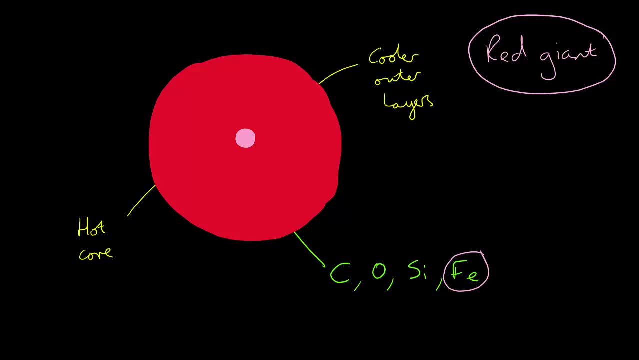 more and more elements until it reaches iron. Iron has got one of the highest binding energies per second. This will happen to our sun in about 5 billion years. When it does, it will engulf mercury and her nucleon. If you want to fuse it into heavier elements, you have to put in more energy than the 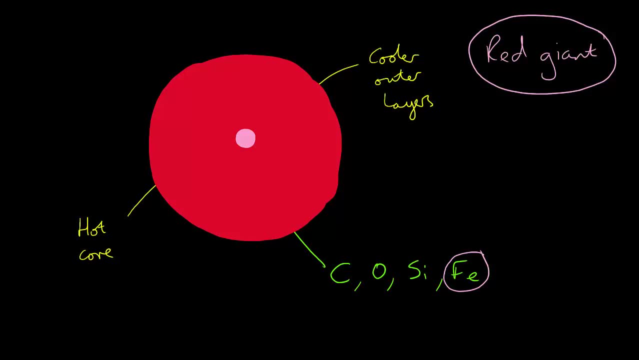 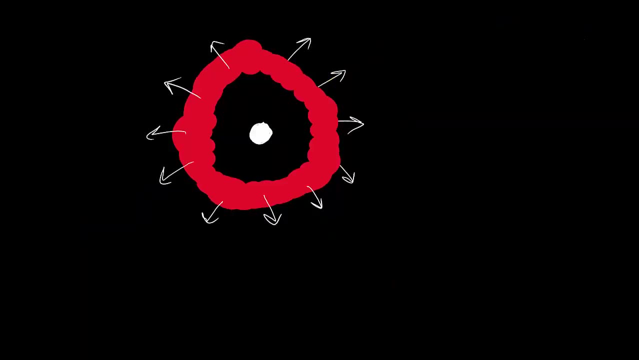 reaction will release. The red giant cannot provide this, so fusion stops again and once more a lack of outward gas pressure will cause the star to collapse. The tenuous, relatively cool outer gas of the star will drift into space as a planetary nebula. Note that planetary nebulae. 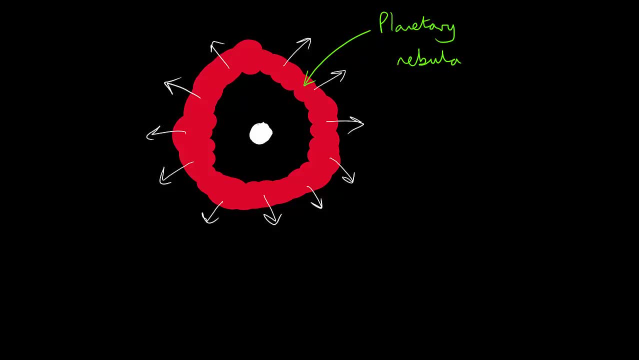 are nothing to do with planets. it's an erroneous historical name that's stuck. If the remaining core of the star has a mass no more than 1.4 times the mass of the sun- and this corresponds to an original star with a mass less than 4 times that of the sun- it will become a white dwarf. 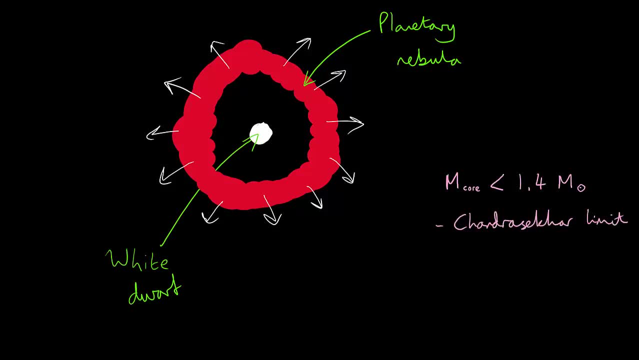 This limit is known as the Chandrasekhar limit and is because below this limit the electron degeneracy pressure prevents further star collapse. The white dwarf is very hot, hence its colour, but it is no longer fusing. It will slowly fade for eternity, like the dying embers of a fire, until eventually it becomes. 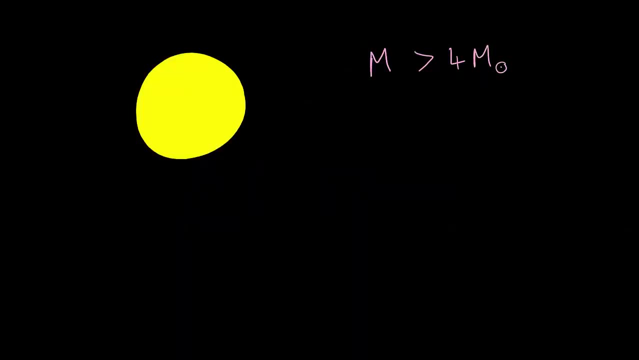 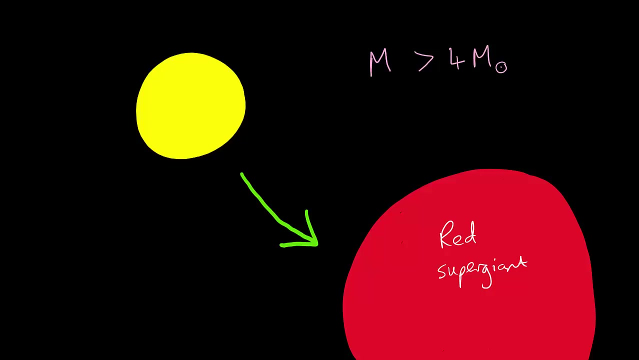 invisible. But what happens to larger stars, Stars with a remnant mass above the Chandrasekhar limit or the original mass, that's, more than 4 times the mass of the sun? Well, their evolution is slightly different, Similar to low mass stars. their core will collapse and they'll begin fusing. 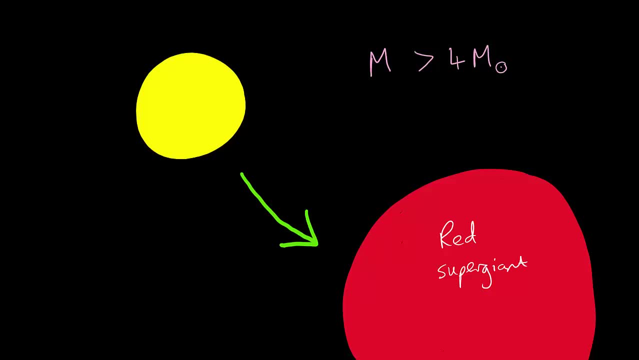 heavier elements, but they'll expand into much larger stars called red supergiants, which can be up to a thousand times the diameter of the sun. When a red giant finally runs out of fusible material, it will also collapse, but the energy 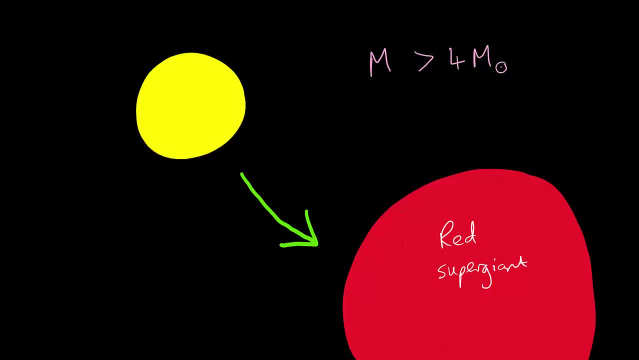 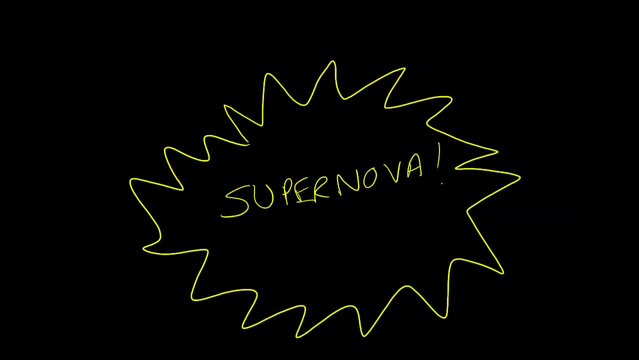 available in this collapse will be so great that even the electron degeneracy pressure of the core cannot prevent further collapse. This causes a supernova, an enormous release of energy which can briefly outshine the hundred billion other stars in the galaxy. A supernova. 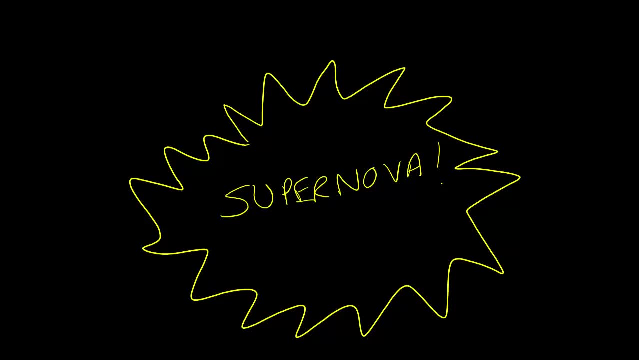 is hot enough to fuse iron into even heavier elements. The fact that these elements are found in our bodies and on the earth mean that we are made of the remnants of a supernova that happened somewhere in this region of the universe long before the formation of our sun and the planet. 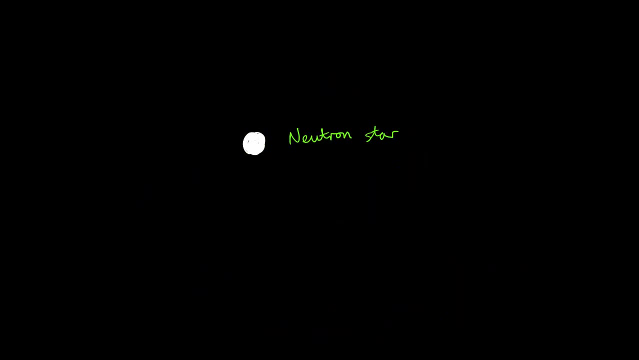 We are quite literally made of stardust. Unless the original star was exceptionally massive, the remnants of the supernova will form a neutron star. A neutron star has collapsed to such an extent that all of the empty space from the atoms has been squeezed out, leaving only the nucleons. 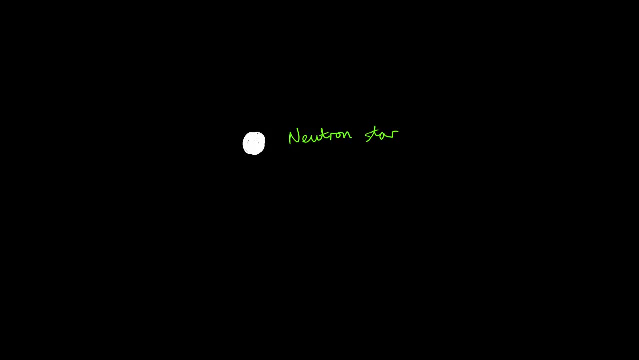 behind. The density of a neutron star is tremendous. One teaspoon of neutron star material has got roughly the same mass as the combined mass of every human on earth. The neutron star is prevented from collapsing any further by the neutron degeneracy pressure. However, 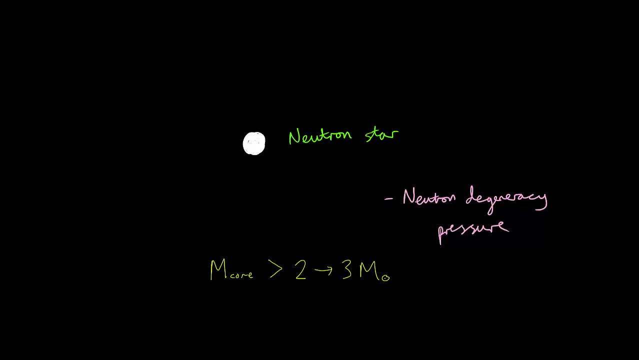 if the star's remnant is more than around two to three solar masses, even this neutron degeneracy pressure will be a huge problem. This is because the neutron star is so dense that it can't be released into the atmosphere. Stars above this limit, which is called the Oppenheimer-Volkoff limit. 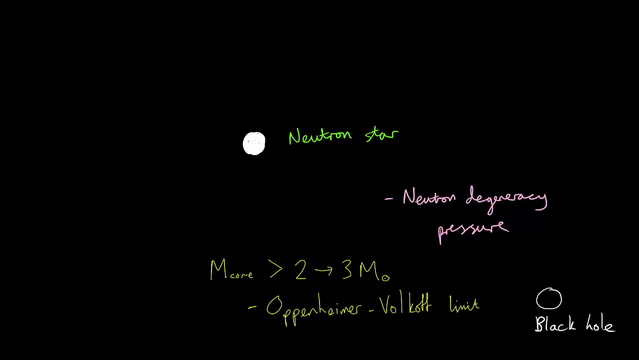 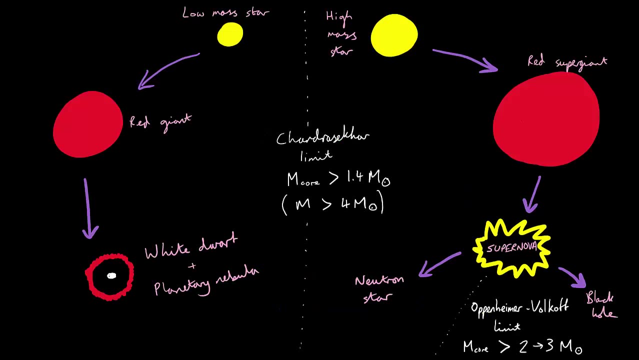 will collapse into black holes. The density of a black hole is so high that it has gravitational effects that prevent even light from escaping. Okay, let's summarise this journey. A low-mass star that is one below the Chandrasekhar limit.